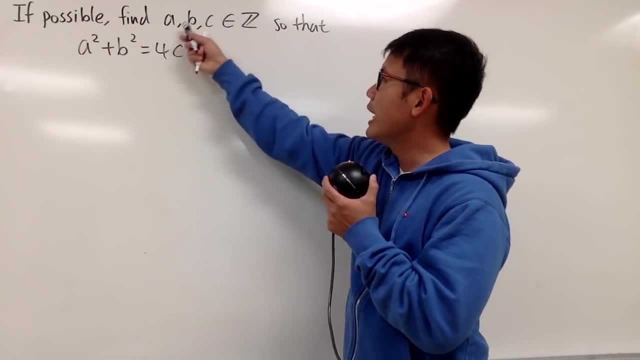 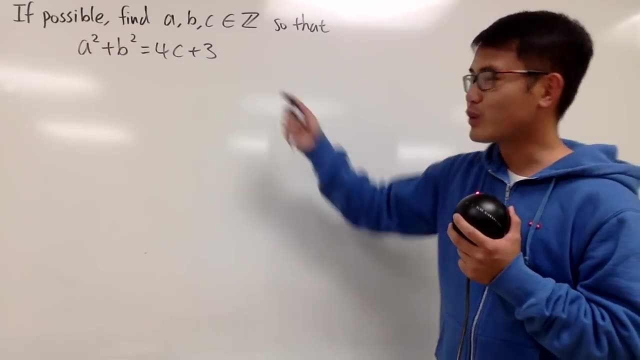 Let's do some math for fun here, If possible. we are going to find integers a, b, c, so that a squared plus b squared is equal to 4c plus 3.. And, as always, please pause the video and try this first. 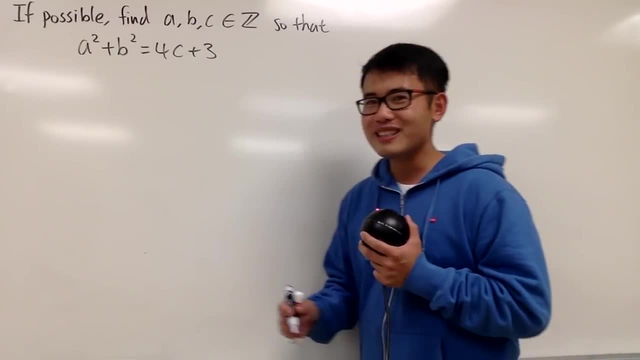 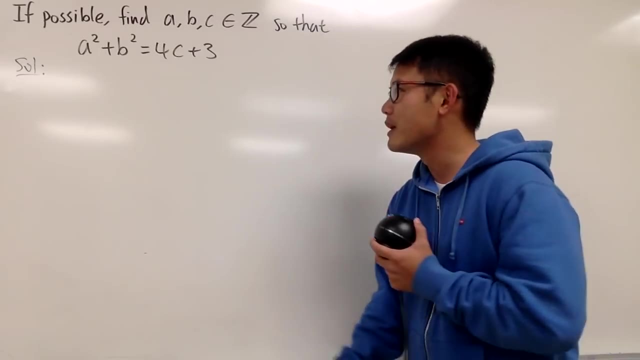 Okay, how did you guys do this, Well? well, let me show you guys my solution right here, And, of course, you should share your solution with us as well. Just leave a comment down below. But anyway, I will show you guys my observations that I'm making along the way. 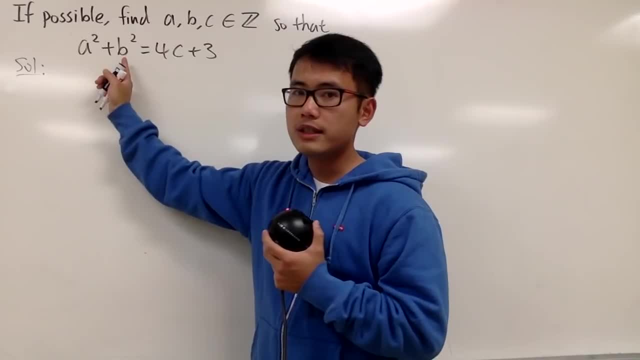 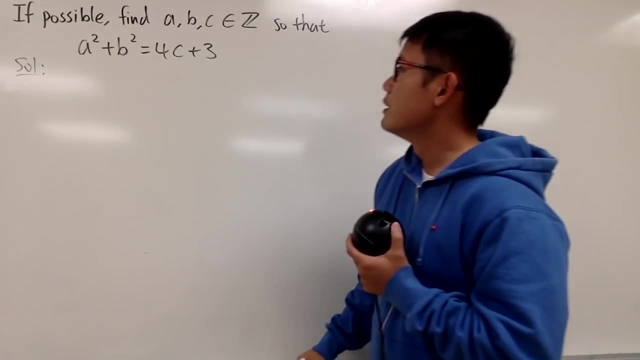 Okay, first of all, we do have a sum of two squares on the left-hand side, So that means this is always going to be greater than or equal to 0, right? So, with that being said, c has to be bigger than 0 as well. 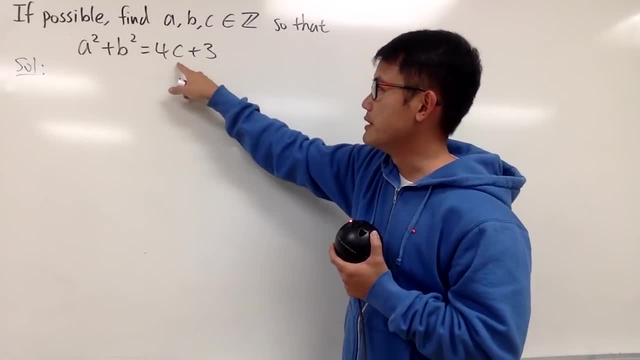 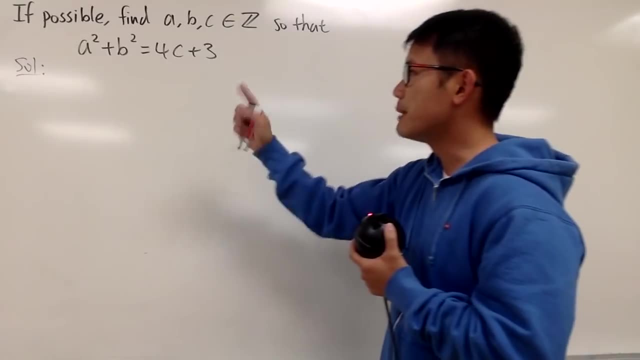 Because imagine, if c is equal to negative 1, then you get 4 times negative 1, which is negative. 4 plus 3 is negative 1. And you'll get a contradiction right, Because it's not possible for you to have a squared plus b squared is equal to negative 1.. 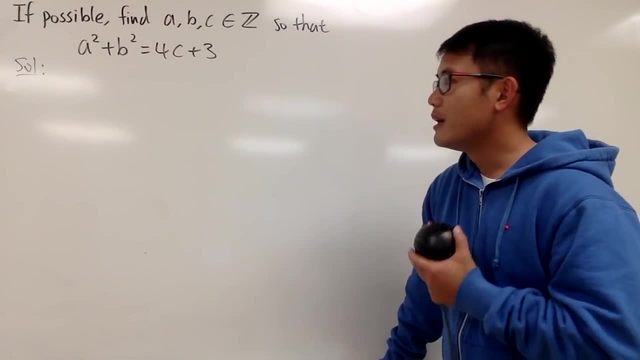 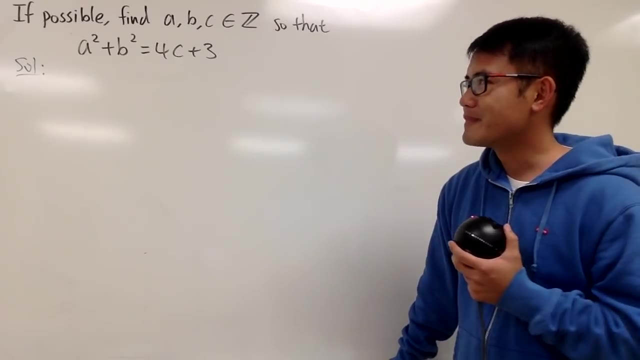 When a and b are just integers, right? So it's not possible. But the truth is that it doesn't really matter if a, b, c are positive or negative, right? Hmm, So that's kind of out of the consideration. 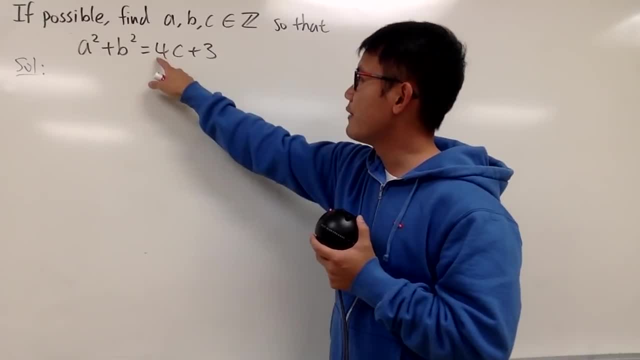 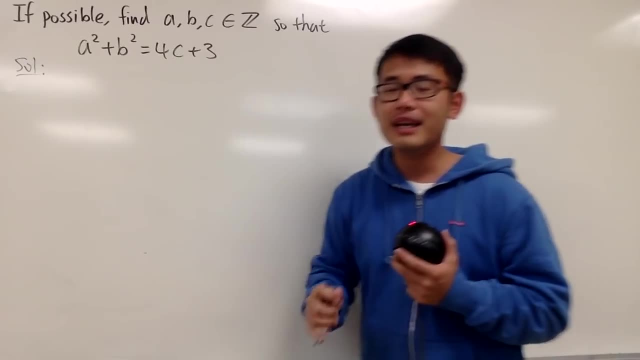 But anyway, let's take a look at the following. Notice that 4 times c- this right here is always even, And when you add 3 to that, the right-hand side is always odd. Sometimes you have to be aware of the even and oddness, okay. 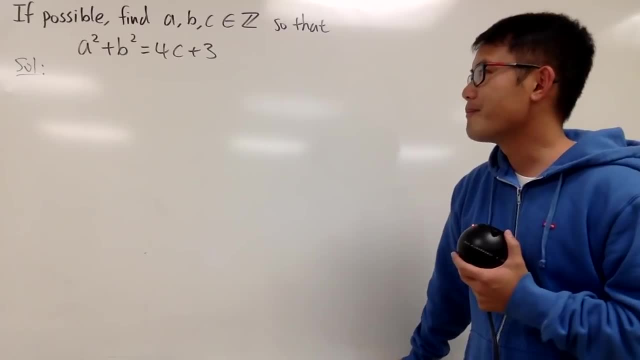 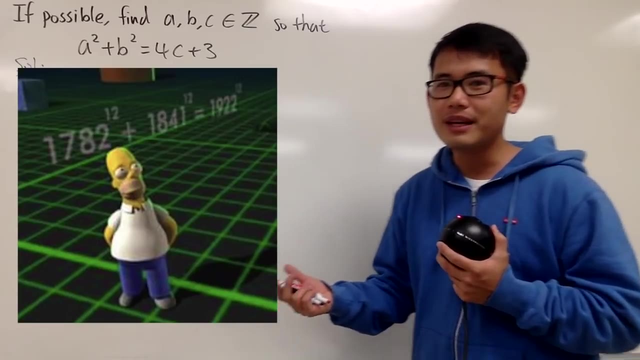 The evenness and the oddness. And um, there is a little proof by the Simpsons. He claimed that he found the counting example to different from last theorem. right, But I can easily disprove his counting example by using the even and oddness. 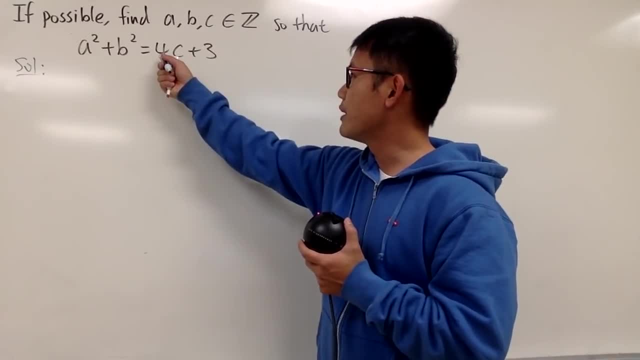 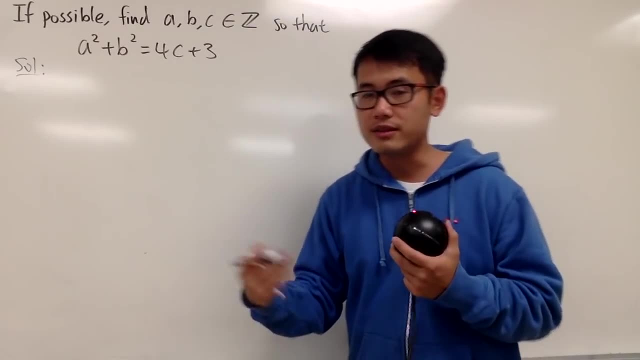 Anyway, here is how we are going to observe. I will just write down. okay, we know 4c plus 3 is odd, And let me just write down all the steps. if you want to write down your solution, this is what you will do. 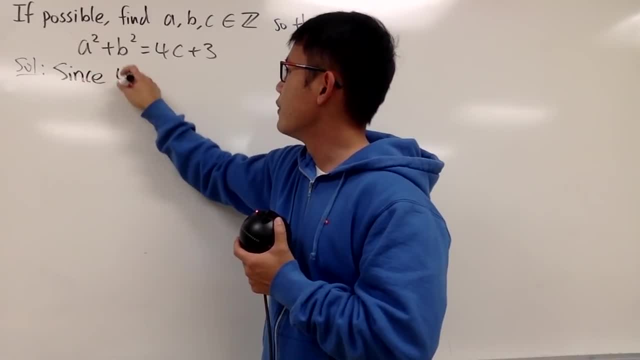 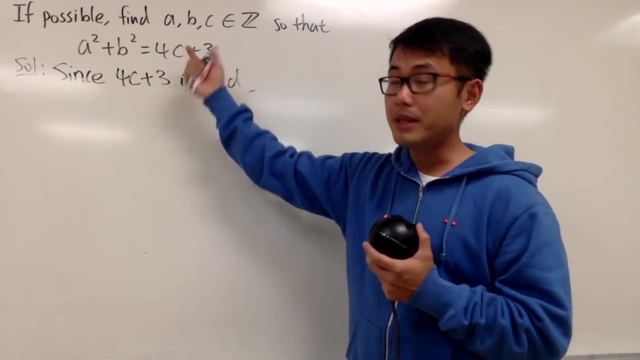 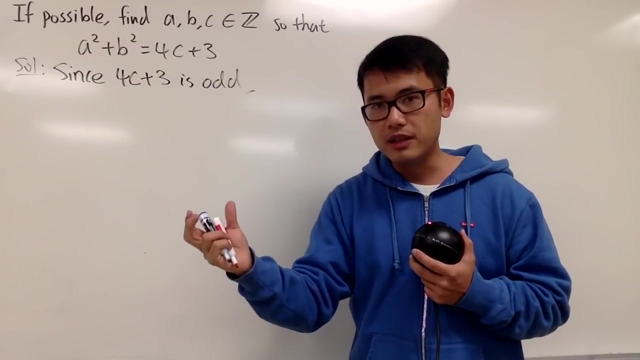 I'll just say, since we noticed that, that 4c plus 3 is always odd, so the right hand side is always odd. What does that mean? Well, when you have one thing plus the other being an odd number, you must have one of them being even and the other one being odd, right? 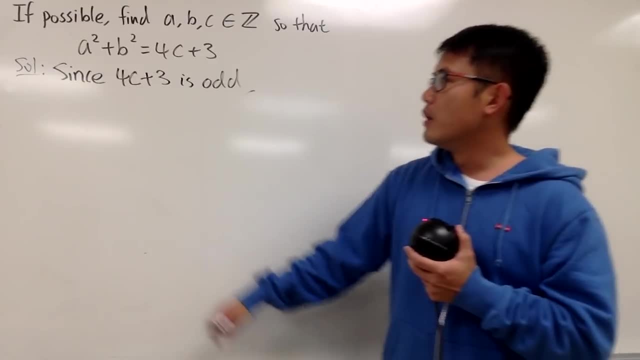 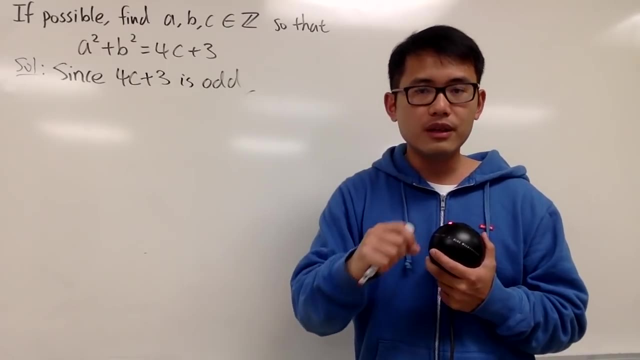 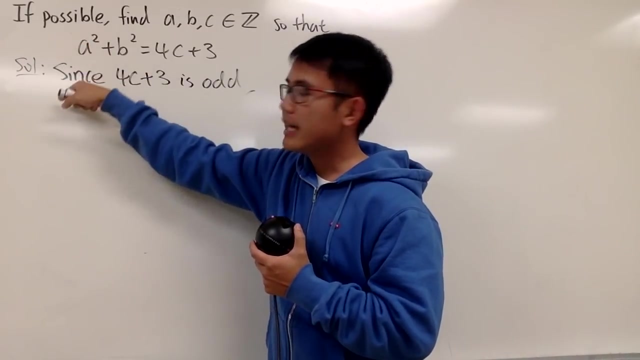 Because even plus odd, it's odd, right? Well, these are just squares of a and b. If you have an even number, you square, that you get even. If you have an odd number squared, you get odd. And if you have a squared being even, a has to be even. 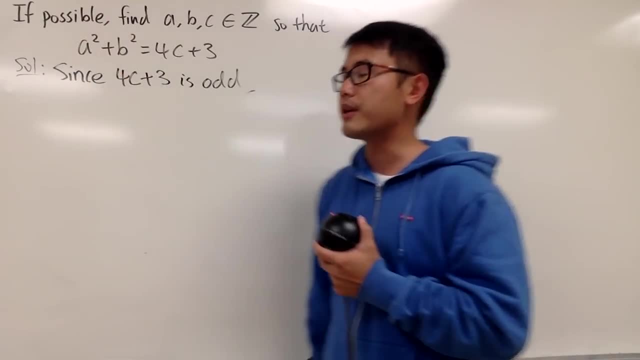 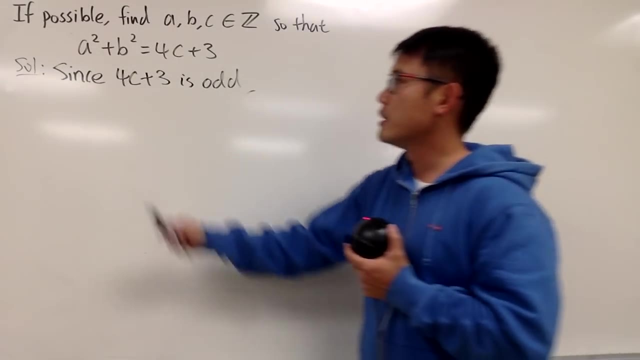 And, for example, if a squared is odd, then that means a is odd. So they go back to back. But anyway, we know that the right hand side is odd. That means either this or that is odd, and the other is even. 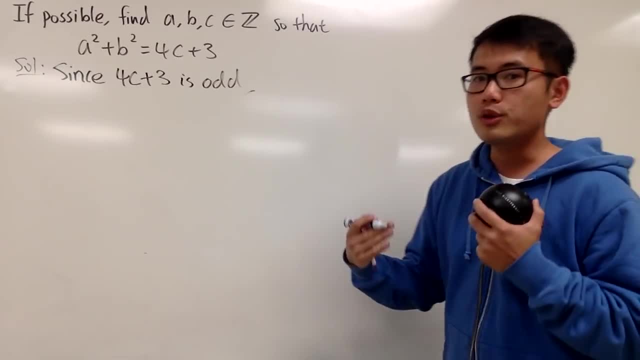 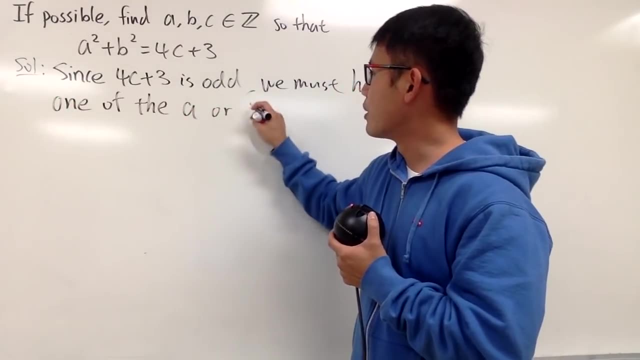 That must be true, And once again we are just going to write down what we just said. So we are just going to say that we must have one of the a or b to be even, And once again I'm just saying a and b. okay. 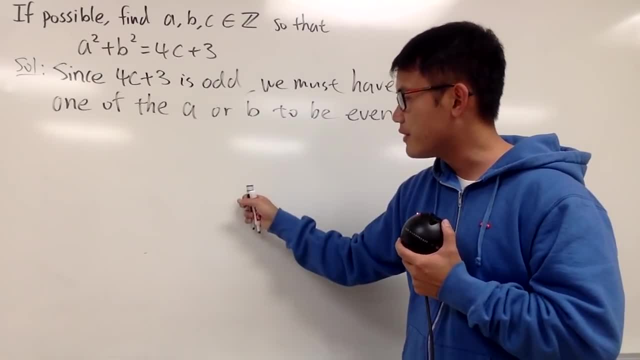 Because, once again, when you have a squared, it's even. That means a is even. When you have a is even. that means a squared is even. So they go back to back And we just want to talk about a and b like this. 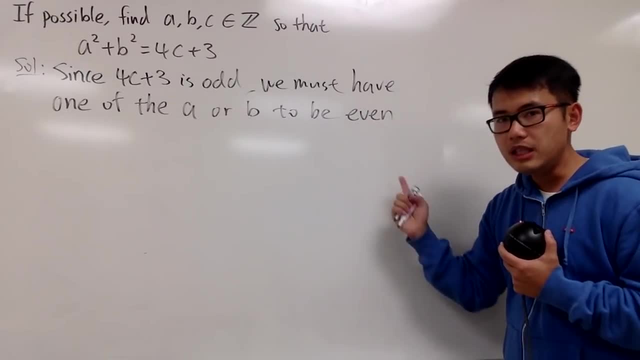 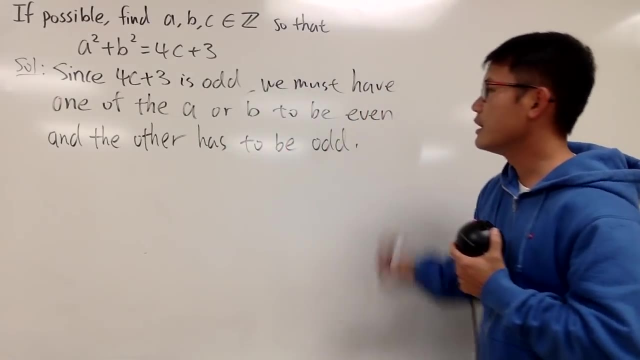 But anyway, I'm saying that either a or b has to be even and the other one has to be odd. Okay, So that's the idea. And now this is what we can do, And this is one of the abbreviations that you guys have seen in the past. 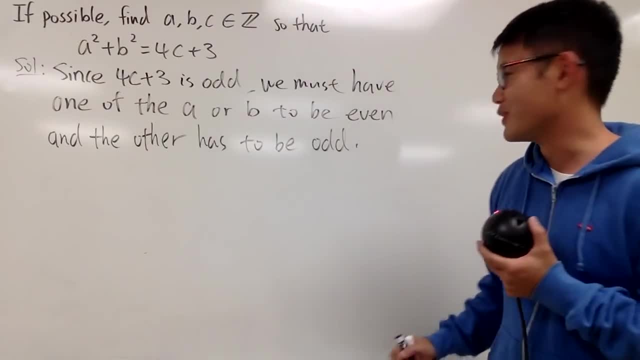 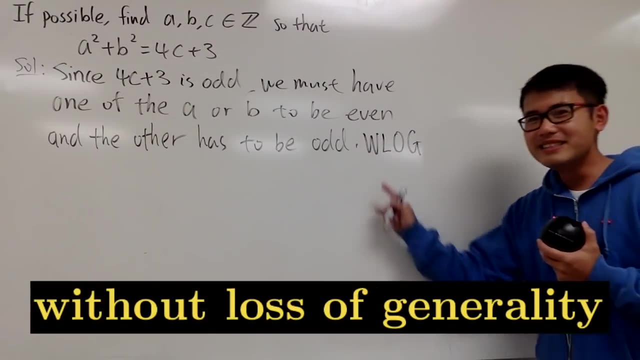 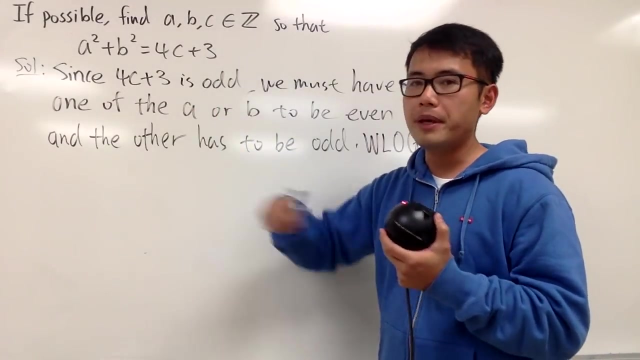 This is the coolest logarithm. No, just a joke. I will just say: without loss of generality. okay, w log, This stands for without loss of generality, And what this is doing is that. well, you don't need to worry about you. pick a to be even. 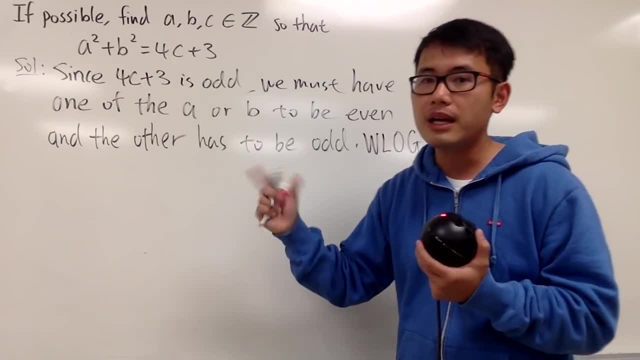 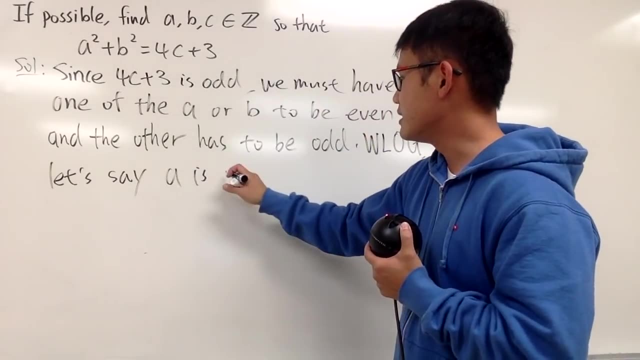 or b to be even, because it's either a or b right, So it doesn't really matter. So I'll just say, without loss of generality, let's say a is. let's just say a is even and b is odd. 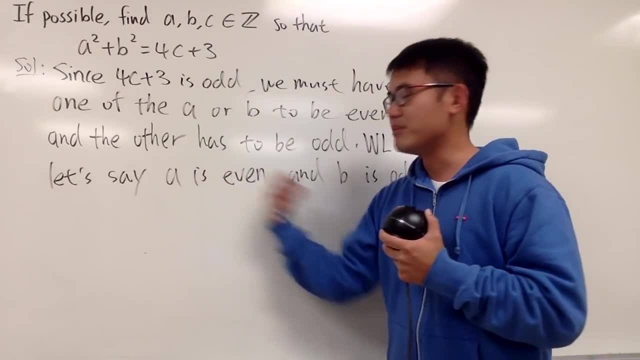 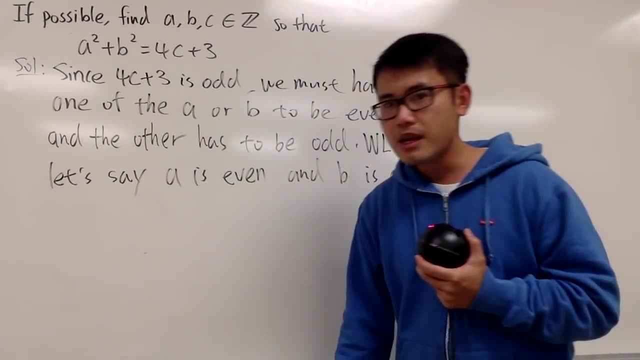 Okay And seriously, you can just change the a and b. You can say a is odd and b is even. That doesn't really matter, But you do put this down so that it can be legit. Okay, so now you know a is even and b is odd. 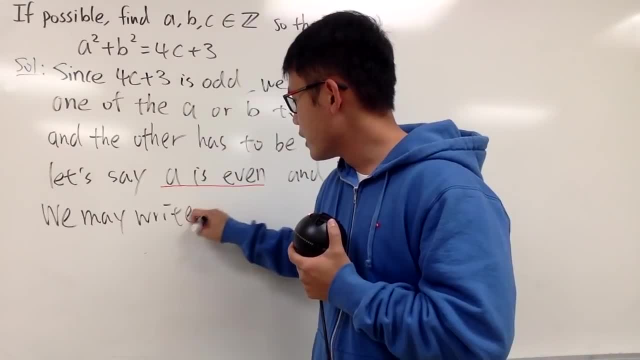 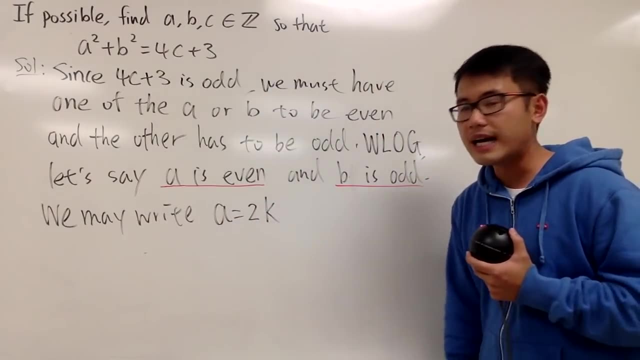 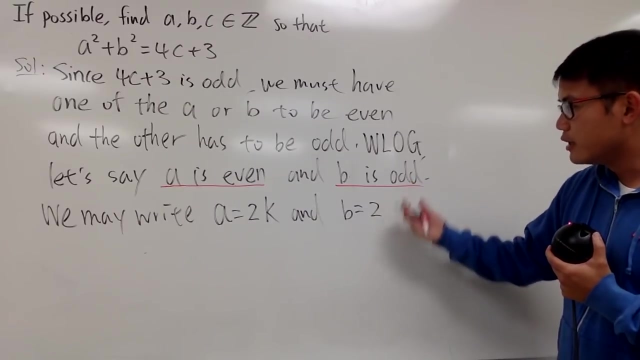 based on what we are saying. right, We may write. when we have an even number, we can say a is equal to 2 times some other integer. I'll just put down k for that. And because b is odd, we can say b is equal to 2 times another integer. 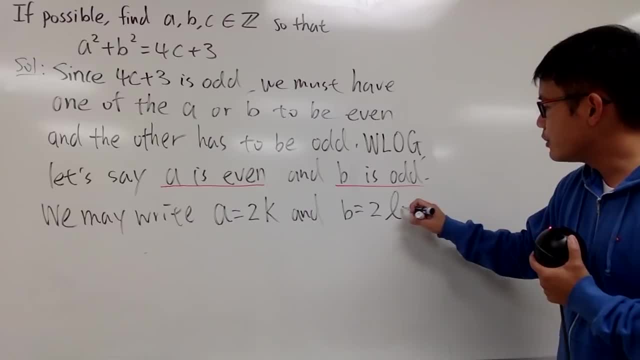 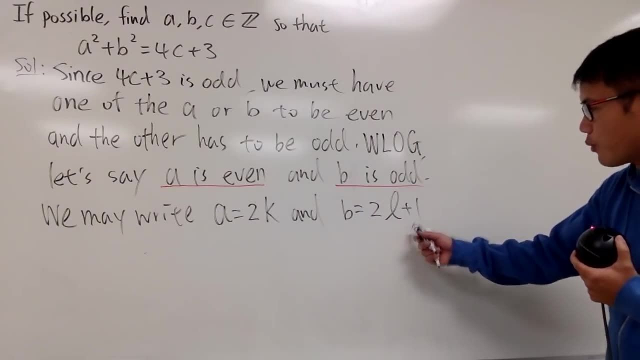 It doesn't have to be the same as k, So we just put down l, But at the end you put down plus 1.. Okay, So this is the form for even number And this is the form for the odd number. 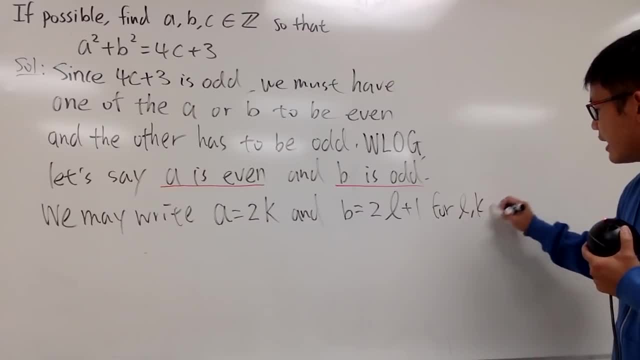 And I will just say for l, l and k be in the integers. This is like a horrible z sorry, But anyway, just like this. okay, So l and k are integers. Now we have an expression for a and b. 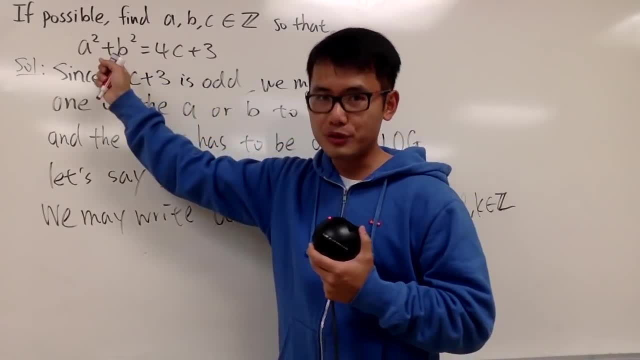 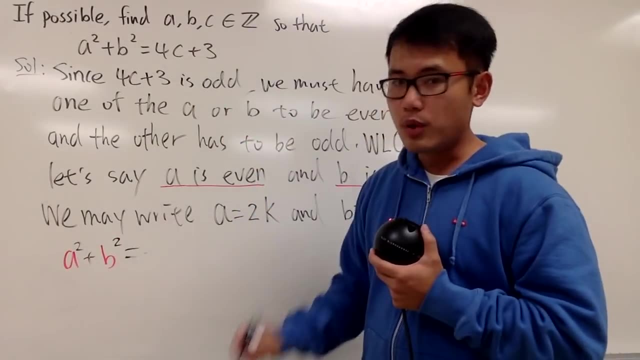 This is what we can do, Of course. we're just plugging this back into the original equation, So we know that a squared plus b squared. now this will be okay. a is 2k, not like the 2k18 for the basketball games. 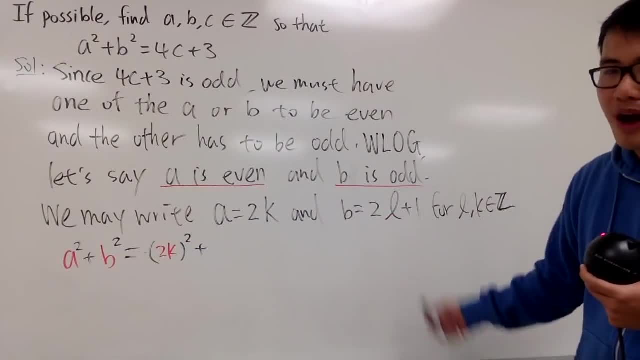 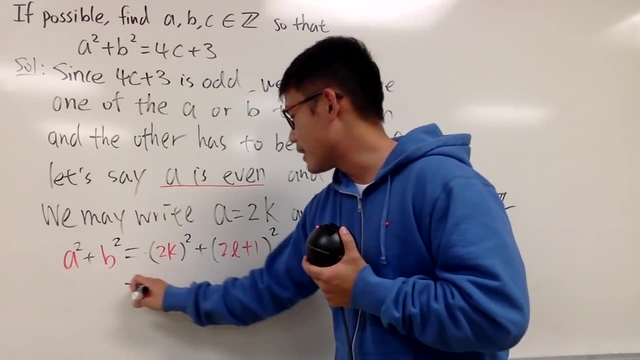 but you know 2k, And then b is 2l plus 1.. So we just add plus 2l plus 1.. Okay, And now we can just do some algebra: 2k squared is of course just 4k squared. 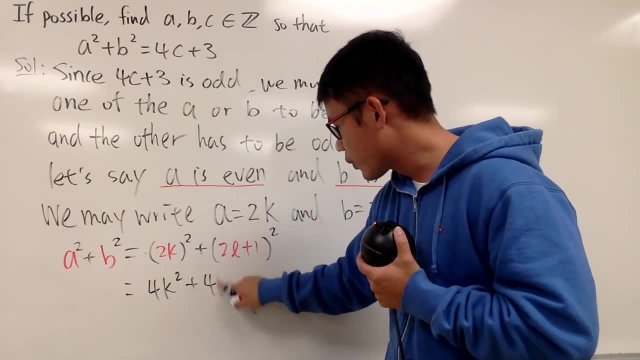 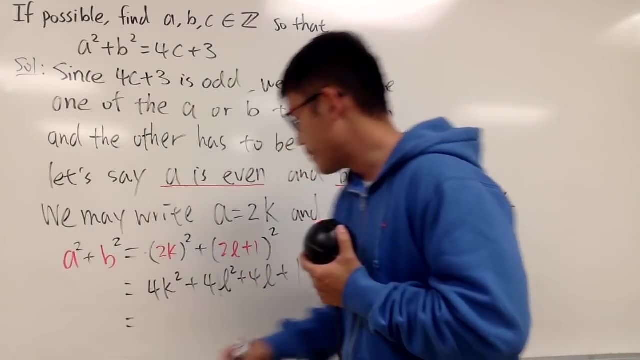 And then when you multiply this out, you get 4l squared plus 4l plus 1.. And here's the part that you have to kind of just pay attention to. Well, notice that the first three terms that we have right here. 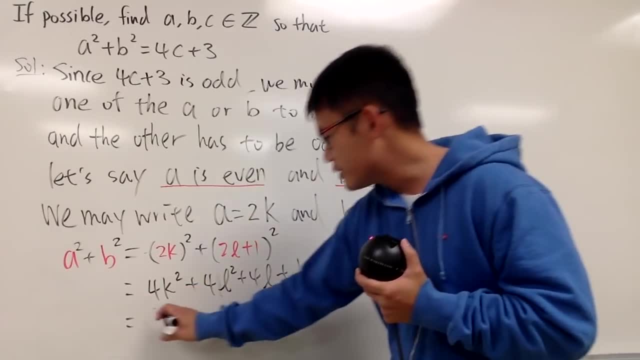 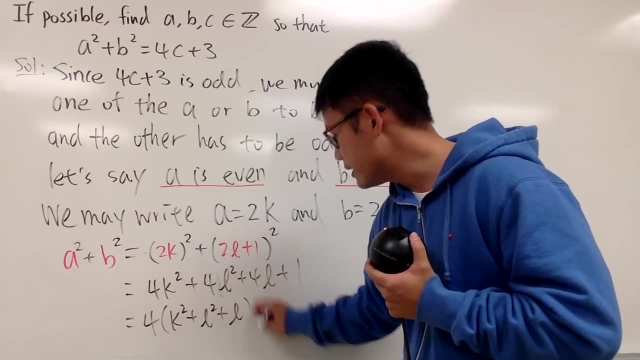 they all have a four times right, So we can factor out the four. So let's do that. This is four parentheses, and we have k squared plus l squared and then plus l, like this, And then we have the plus 1 after that. 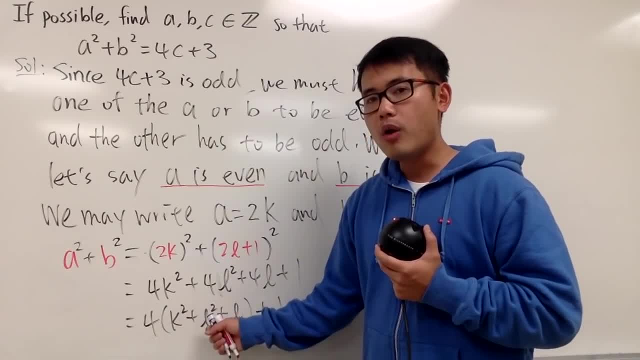 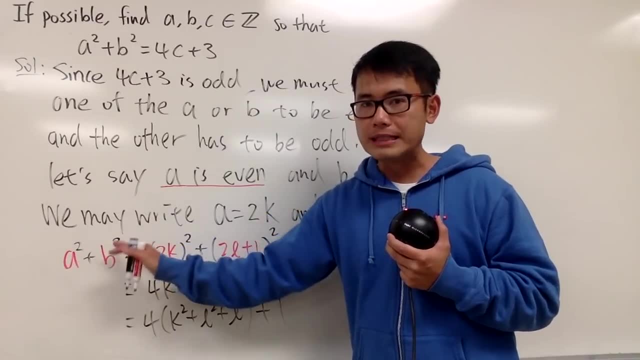 And now take a look: k and l are integer, So right here, this must be an integer, right. So when you have a squared plus b squared, notice the four has to be four times the integer, and then plus 1.. 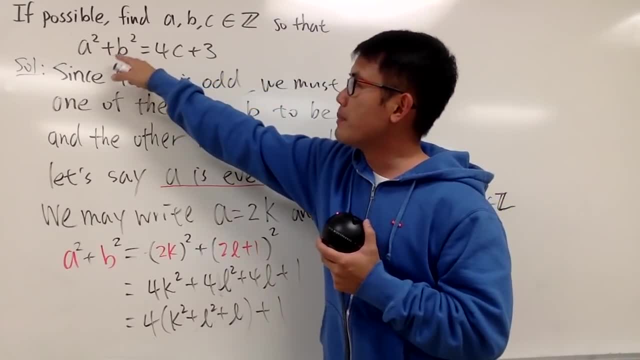 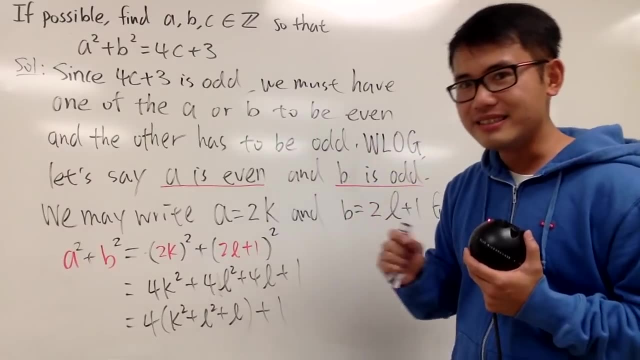 But on the right-hand side this is saying a squared plus b squared, the four has to be 4c plus 3, right, Four times the integer plus 3.. And this is the contradiction. So what we can do is 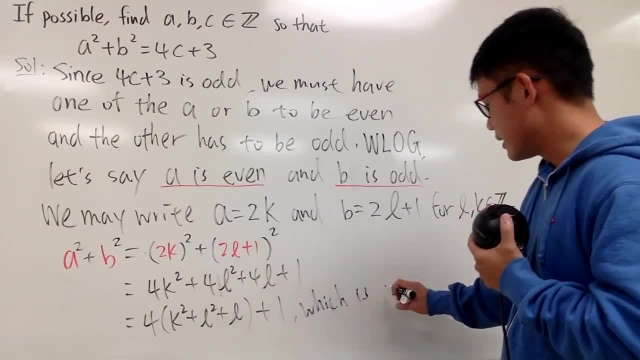 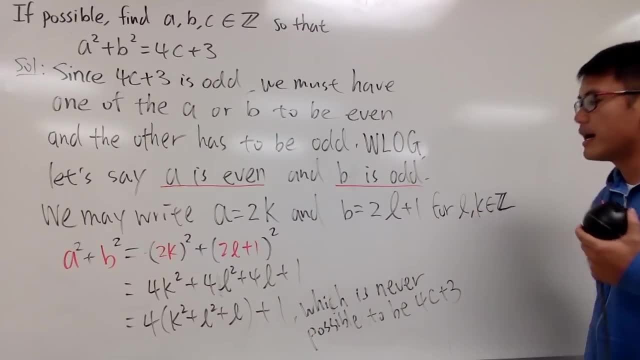 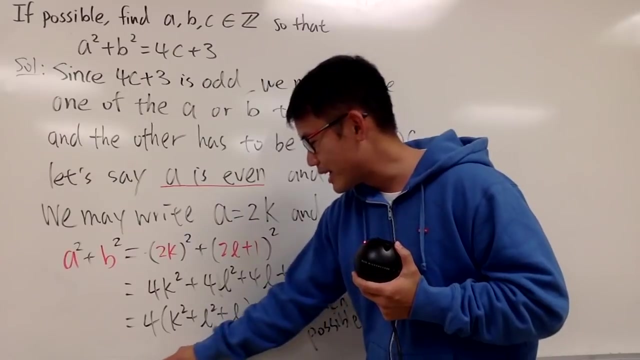 I can just tell you this right here: which is never possible to be 4c plus 3, right, Because once again, you can also use a modulo arithmetic if you want, okay. So if you want to do that, 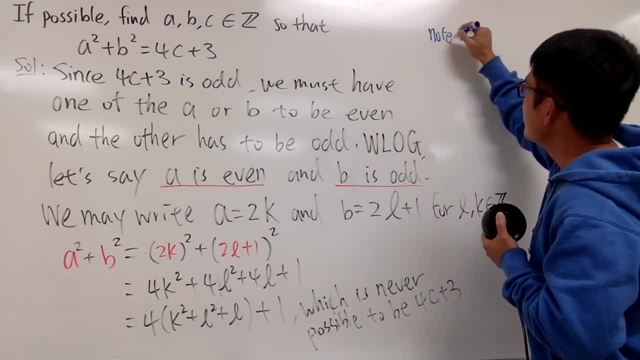 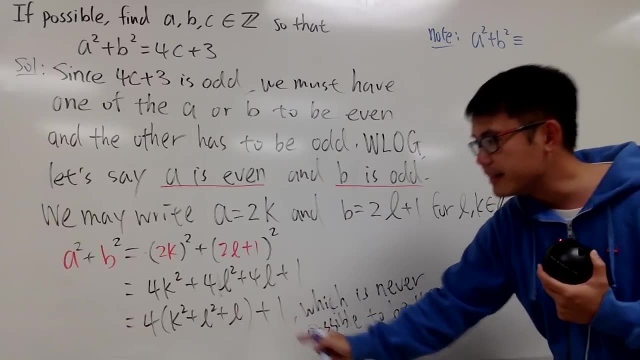 you can say the following right here. Another way to write it, you can say that a squared plus b squared. this right here, it's congruent to 1 mod 4, because this part is the multiple of 4, and then, when you divide this by 4,, 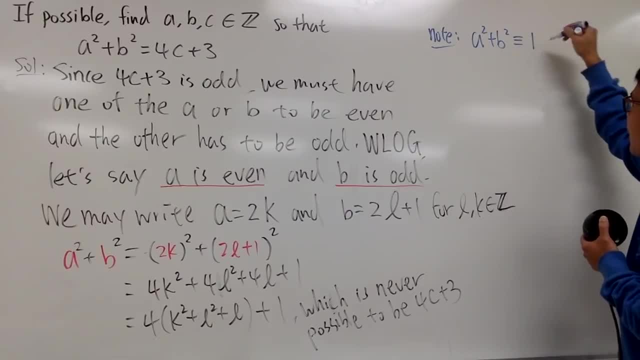 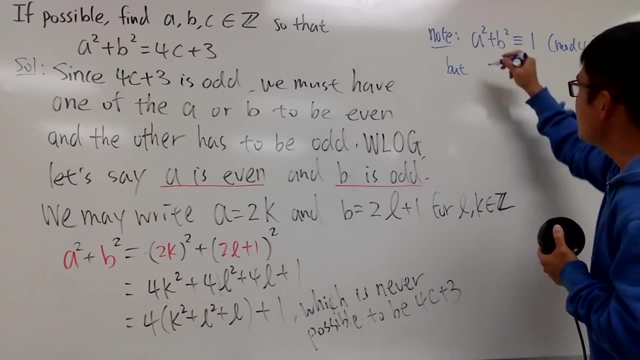 you get a remainder of 1, right. So you can say this is congruent to 1 mod 4, but when you have 4c plus 3, this right here is of course congruent to 3 when you mod 4, right. 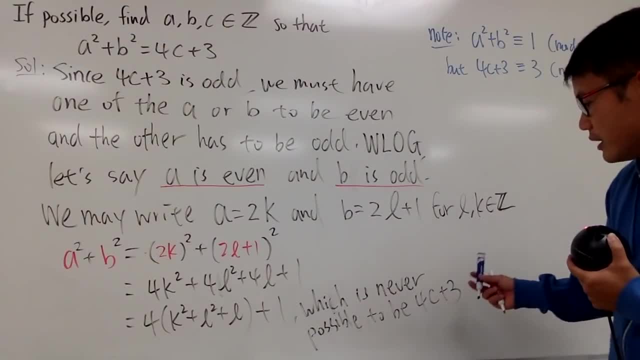 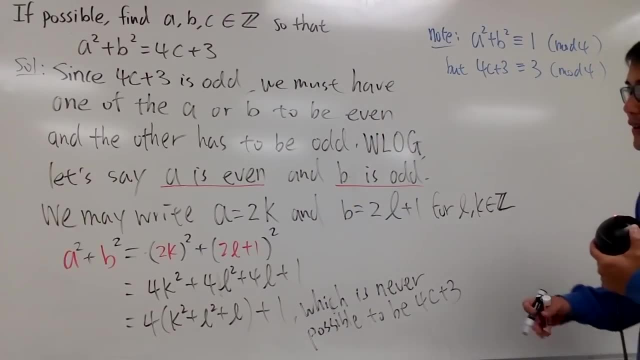 So that's why I said this right here: it's never possible to be the same as 4c plus 3, right When you're talking about just integer solutions. So the idea of all this is that this is actually not possible. 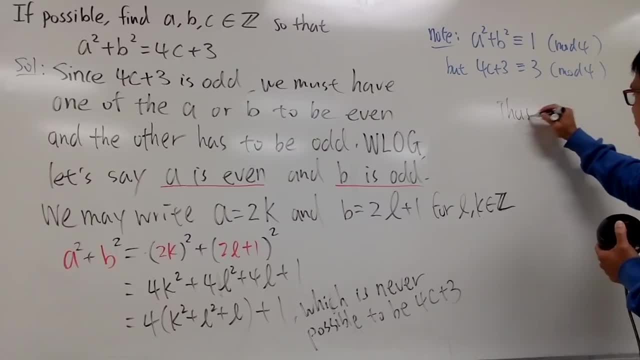 I'll just say it here, you guys that thus let me just write down: we conclude that the equation a squared plus b squared is equal to 4c plus 3, has no inter. technically it's integral solution. but you know, I don't really understand why people say integral. 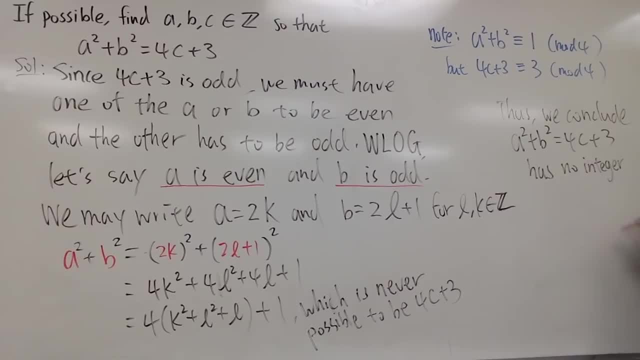 because integral means integral. but you know what I mean. I'll just say: no integers solutions, right, Yeah? so this is how you can do like an argument: oops, I put a box the wrong way, But yeah, I should put a box like this: